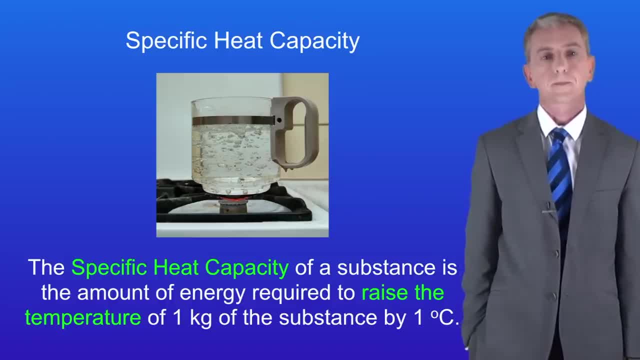 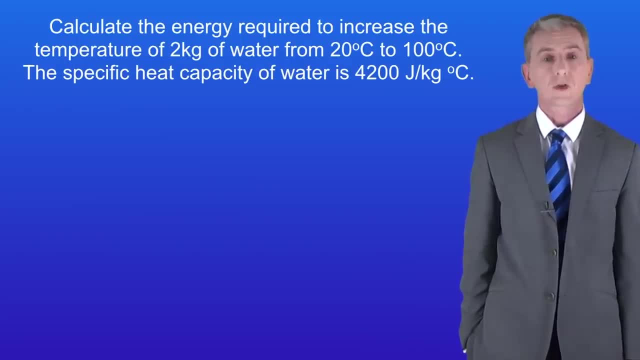 straightforward. So let's take a look at a sample question. Calculate the energy required to increase the temperature of two kilograms of water from 20 degrees celsius to 100 degrees celsius. The specific heat capacity of water is 4200 joules per kilogram per degree celsius. 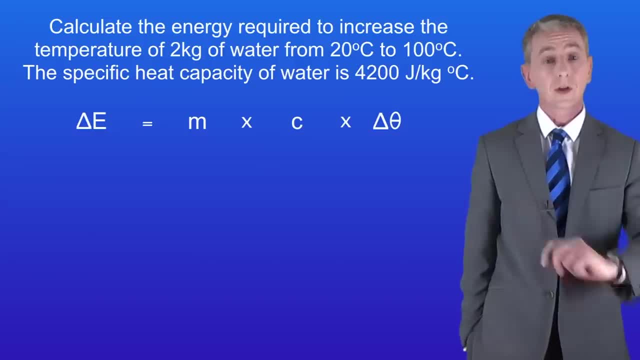 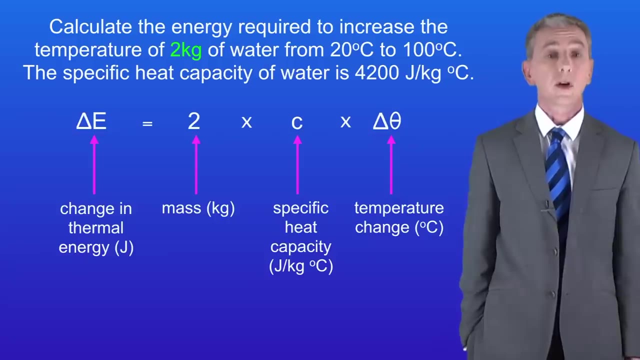 To answer this question, we've got to use this equation and you are given this in the exam. The change in thermal energy in joules equals the mass in kilograms multiplied by the specific heat capacity. multiplied by the temperature change in degrees celsius, We've got two kilograms of water. 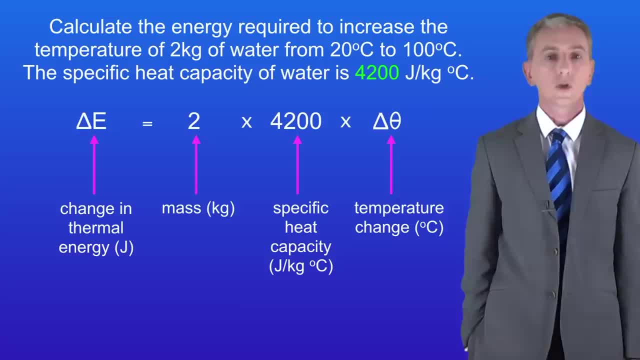 The specific heat capacity of water is 4200 joules per kilogram per degree celsius, and you will be given that value in the exam. and finally, the temperature change in this case is 80 degrees celsius. Putting these values into the equation gives us a total change in thermal. 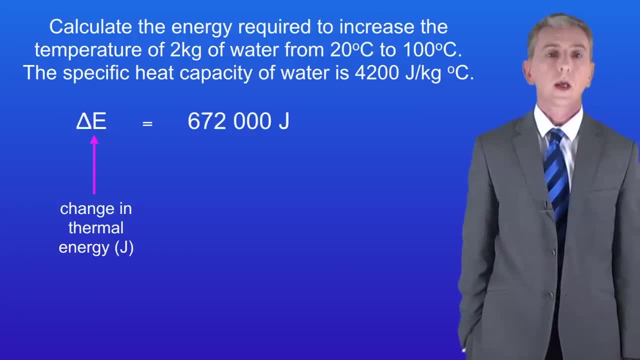 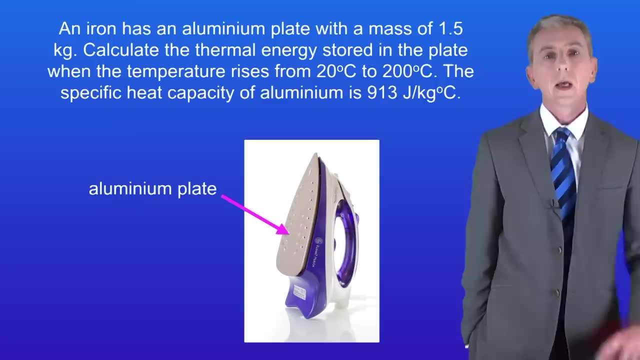 energy of 672 000 joules. We can convert that to kilojoules by dividing by 1000, giving us 672 kilojoules. Here's a question for you. An iron has an aluminium plate with a mass of 1.5 kilograms. 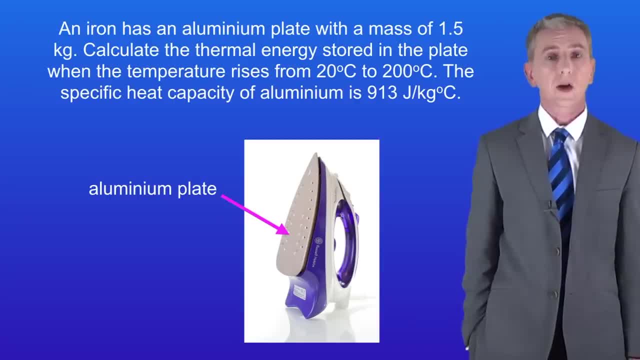 Calculate the thermal energy stored in the plate when the temperature rises from 20 degrees celsius to 200 degrees celsius. The specific heat capacity of aluminium is 913 joules per kilogram per degree celsius. Pause the video and try this question yourself. 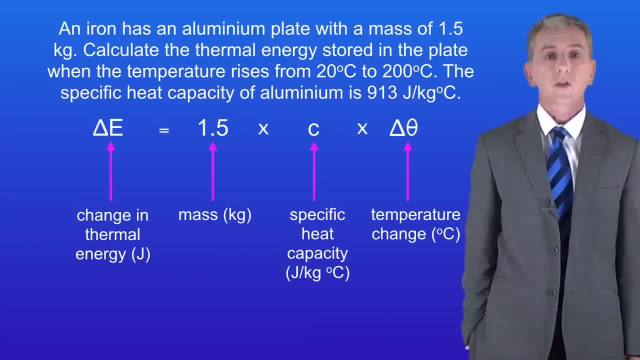 Okay, so we've got a mass of 1.5 kilograms. The specific heat capacity of aluminium is 913 joules per kilogram per degree celsius, and the change in temperature is 180 degrees celsius. Putting these into the calculation gives us a total change in thermal energy of 246 000. 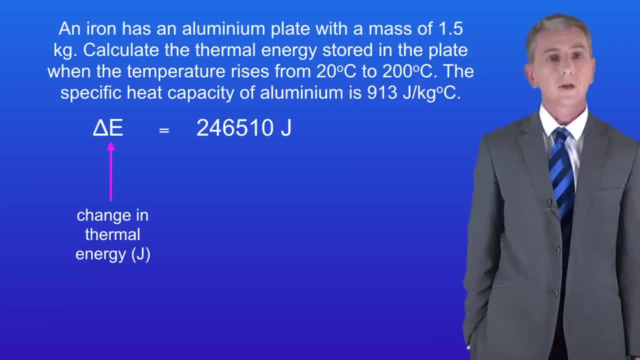 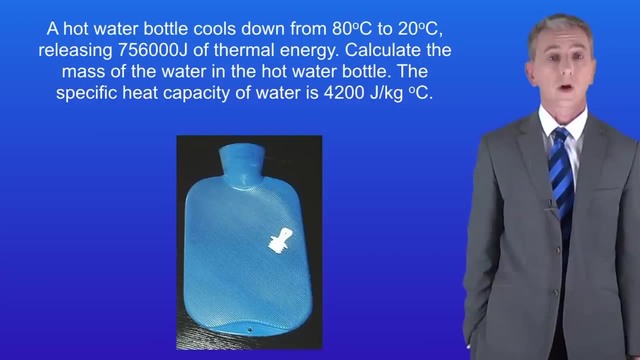 to 510 joules. We can also convert that to kilojoules, giving us a value of 246.51 kilojoules. Here's a final question for you: to try, A hot water bottle cools down from 80 degrees celsius. 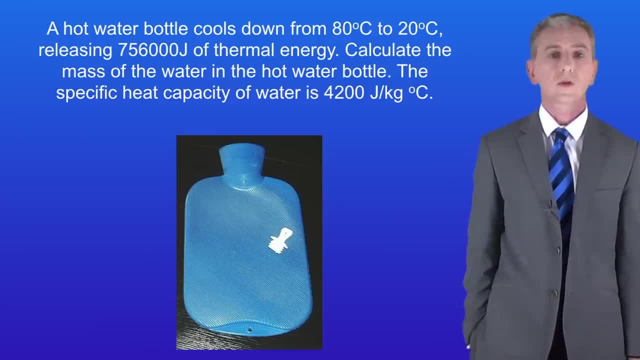 to 20 degrees celsius, releasing 756 000 joules of thermal energy. Calculate the mass of water in the hot water bottle. The specific heat capacity of water is 4200 joules per kilogram per degree celsius. Now to answer this question, you're going to have to rearrange the equation to find the mass.